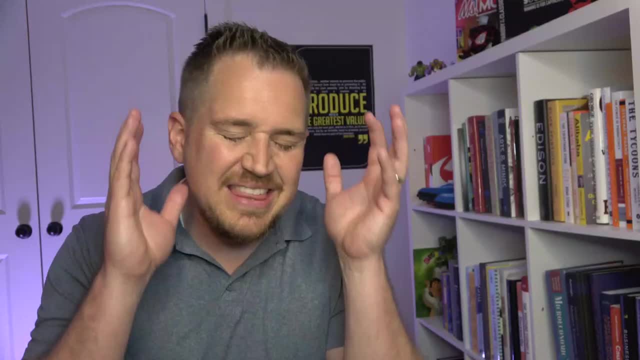 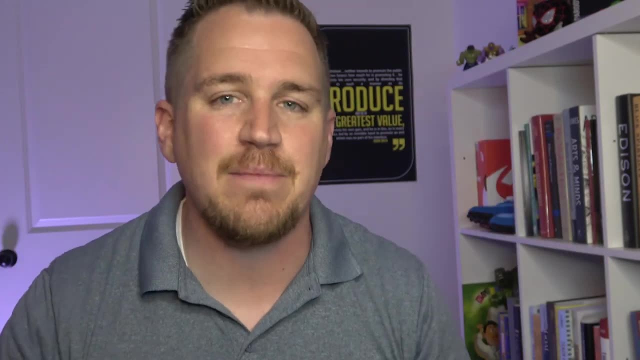 trends and patterns, and then there's also going to be microdata. But this is the type of stuff that you need to use when you're getting started in research, and it comes in and bulks up just about any project you're working on. First, let's get back to FRED. FRED stands for Federal Reserve. 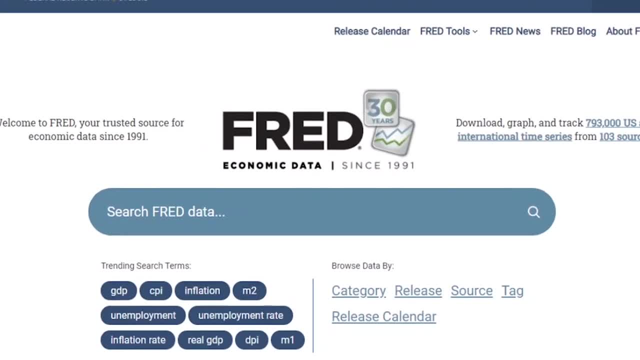 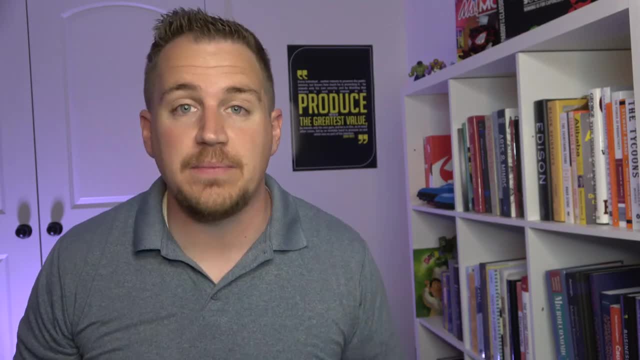 Economic Data. This is a website maintained by the Federal Reserve Bank in St Louis and tracks economic data. When I'm teaching intro economic concepts, I love pulling up this website And just showing people the trends that are here. If you want to look at unemployment since the 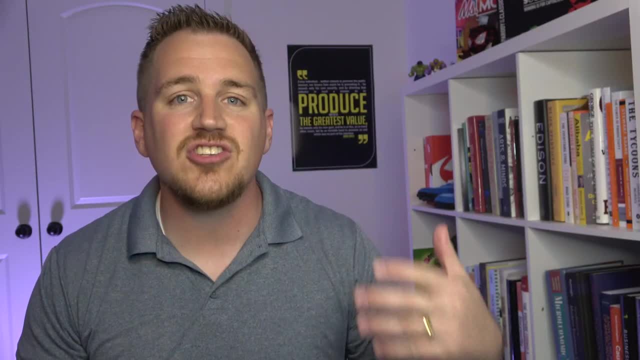 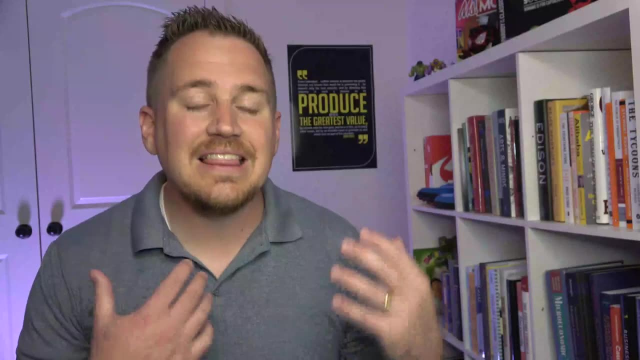 1940s. you're going to be able to find it on this site. But it's not just common economic indicators that you would think of. You can also find the price of chocolate chip cookies since 1980.. I love using this data to just get a big picture idea of what's going on and trying. 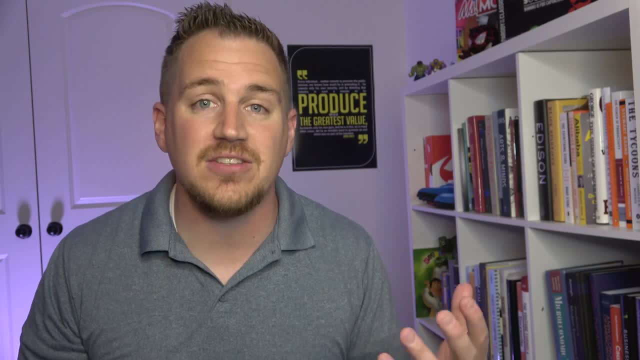 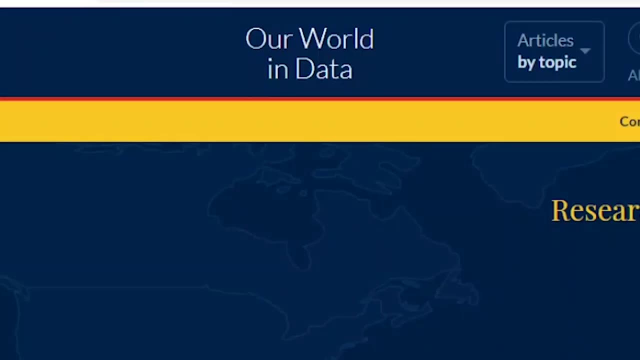 to understand where there might be some interesting trends or patterns that I could dive into and research more fully. The second place where you can go get data is Our World in Data. This is a newer website. It's called Our World in Data. It's a website that's been around for a long time. 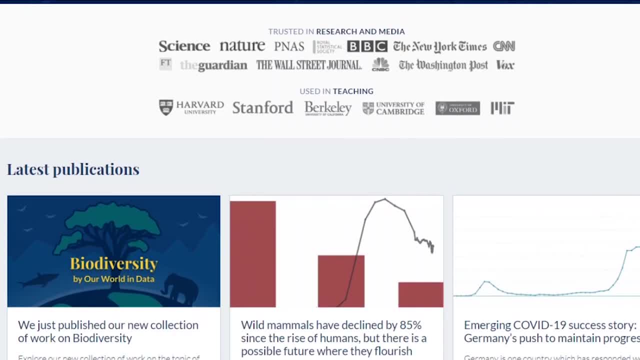 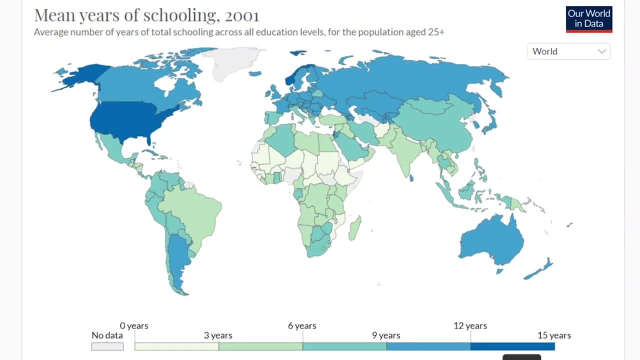 And it's dedicated to tracking progress- just human progress, across time and across space. So you're gonna look at these trends all over the world. you're gonna be able to see where we've made significant improvements and also places where we need more work. There's just fascinating. 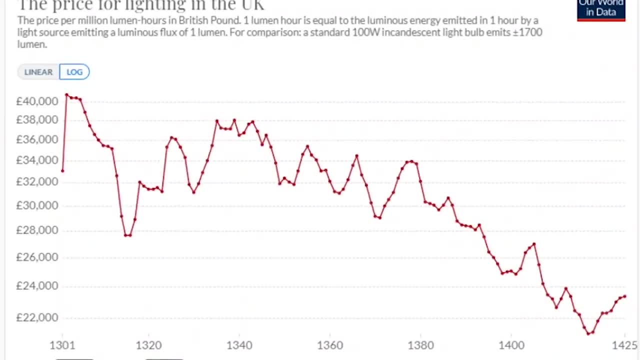 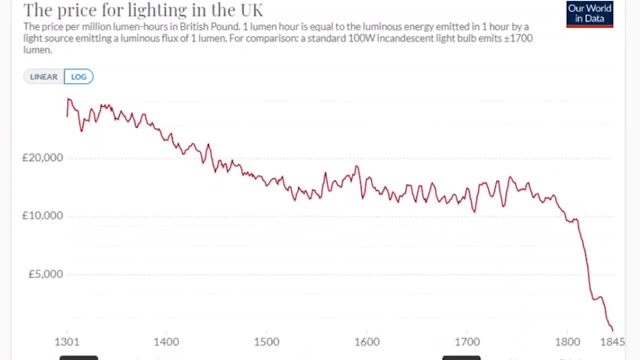 data sets here. Some of them are quirky. I really liked this data set on the price of light over time, where you can see it's very expensive since 1200. And then it declines rapidly as we get into the Industrial Revolution. And then it declines rapidly as we get into the Industrial Revolution. 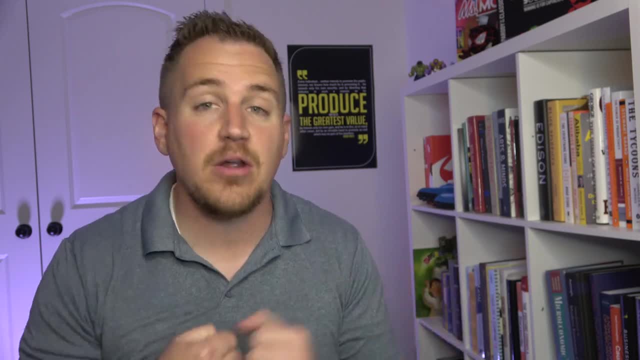 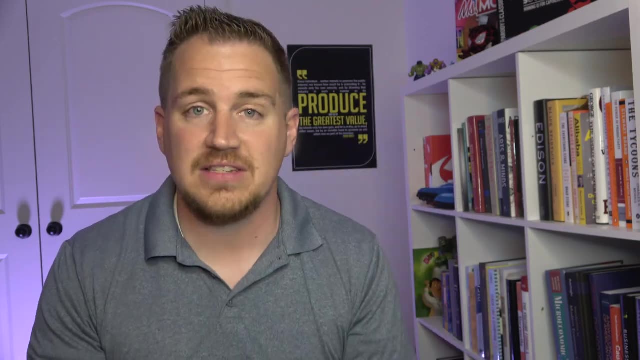 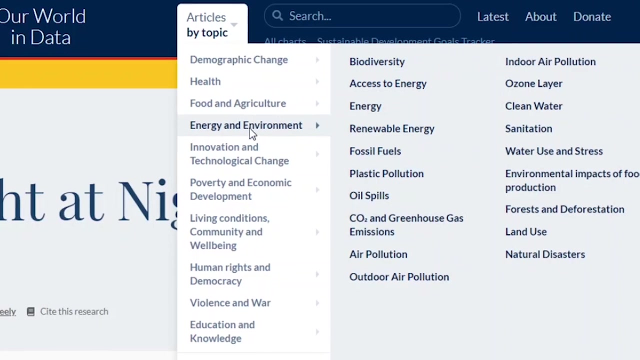 A lot of this is being pulled from academic, peer reviewed sources, it's being pulled from public data sets and it's being collected in a way that you can see progress in the world. So if you're interested in doing anything with human progress- like health, education, conflict, so many other- 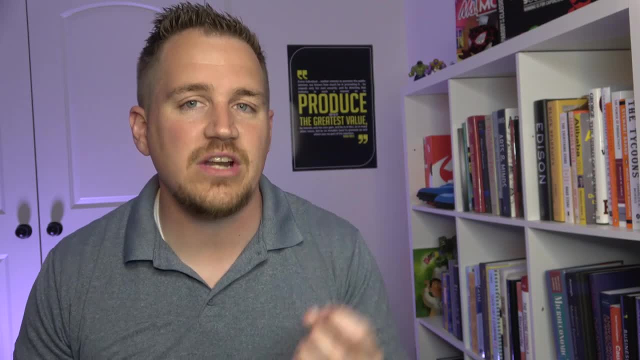 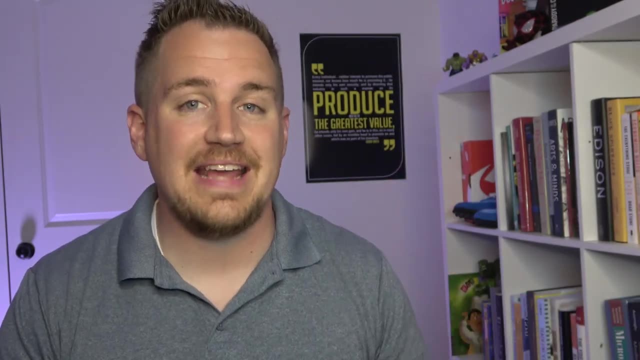 indicators. you can find them in here and you can find some rich resources that you can download and use to motivate some of your economic research. The third data set is the World Bank Database. The third data set is the World Bank Database. The third data set is the World Bank. 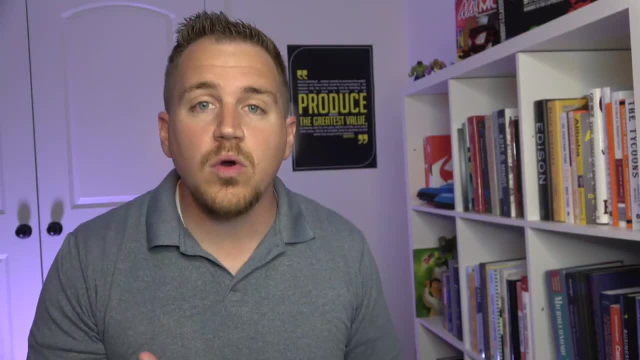 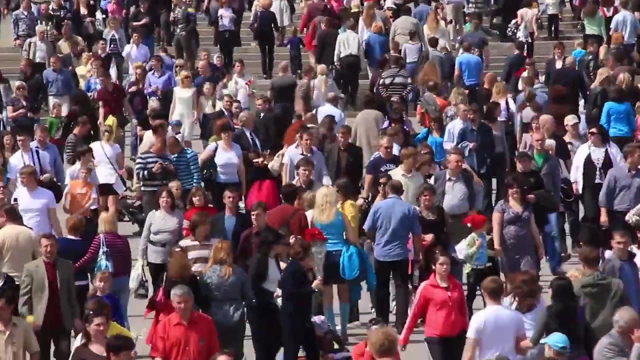 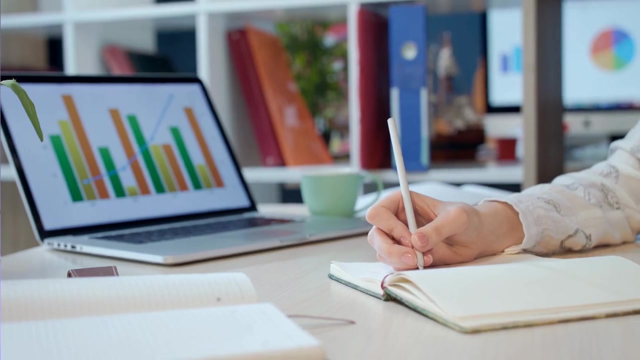 Database. This is a little similar to Our World in Data. Our World in Data is very outward focused in terms of trying to help just the general public get access to economic indicators. The World Bank Economic Data is available for the public, but it's more geared towards researchers like yourself. 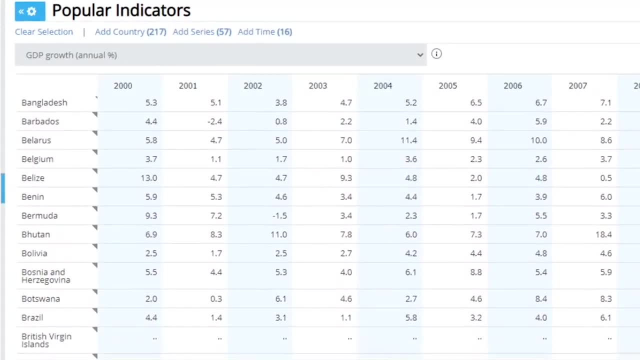 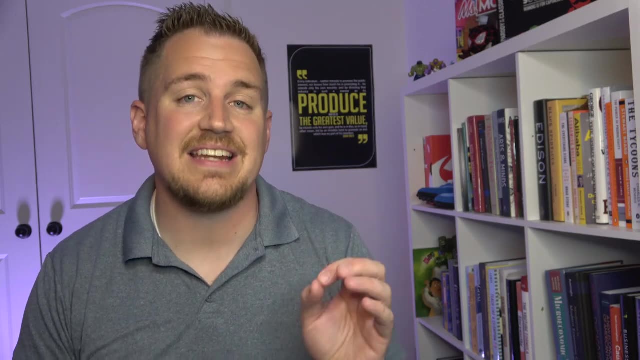 It's just like Fred. I pull in that World Bank data anytime I want to motivate to my students the importance of economic development. So those are my three go to data sets that I use to find progress and patterns, And this can be really helpful when you're thinking of research questions. 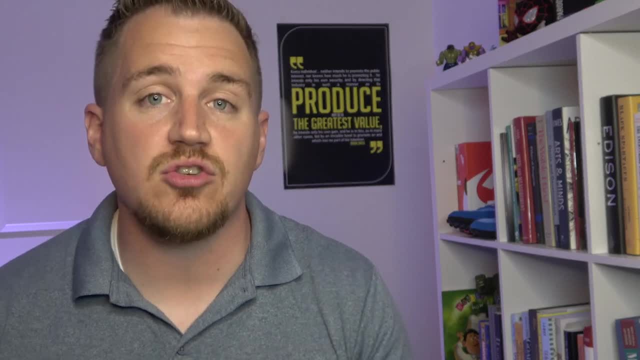 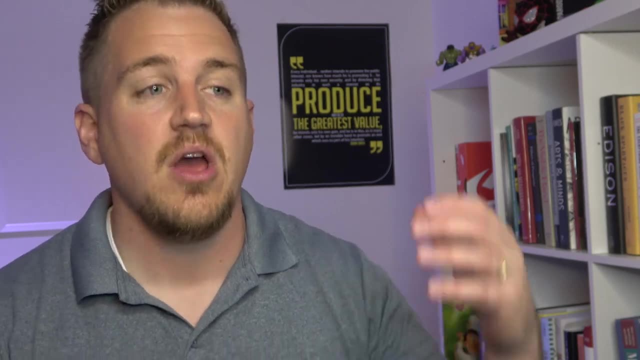 or another thing might be how it motivates your research. Maybe you have a research question that you know is interesting, but you need a little bit more narrative to get people interested in that question. But the trends and these patterns aren't really going to deliver on what you need. 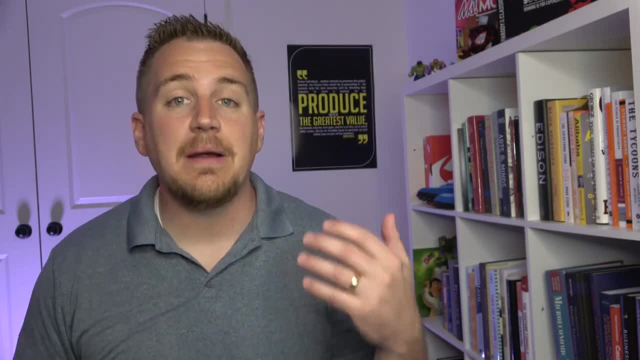 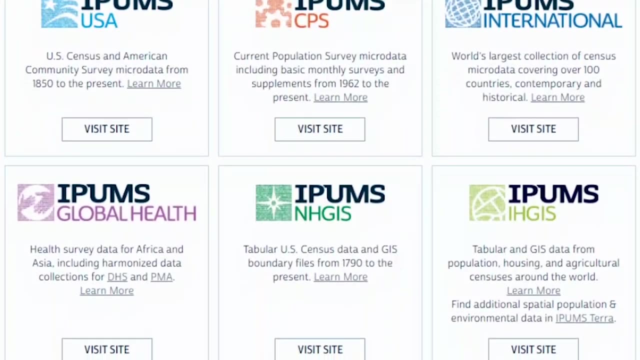 to give a solid answer to these questions. That's when you need microdata. Well, I have three main sources for microdata as well. A classic data set is Ipam. You can go on here and find so many different microdata sets. You can find census data where 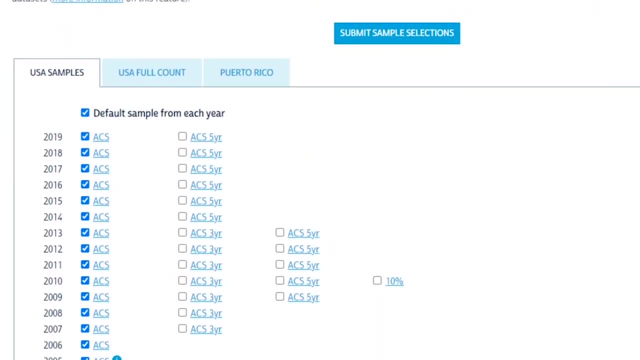 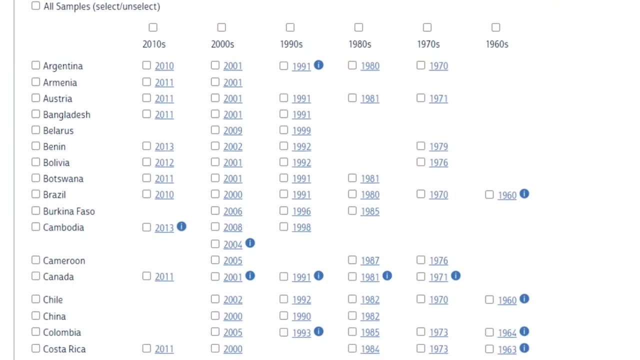 you're going to look at samples of the United States and you can see what's going on with households in the United States. You could go international. You can look at census observations from different countries all over the world- One of the most interesting data sets on here. 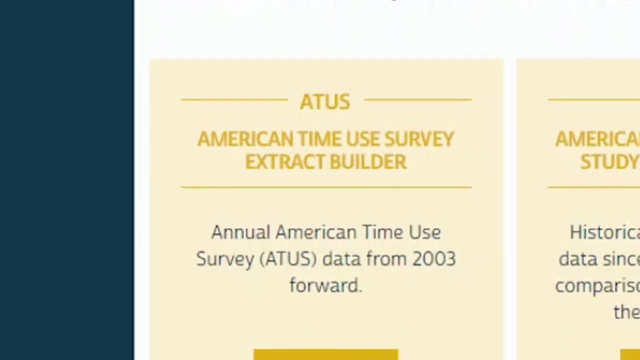 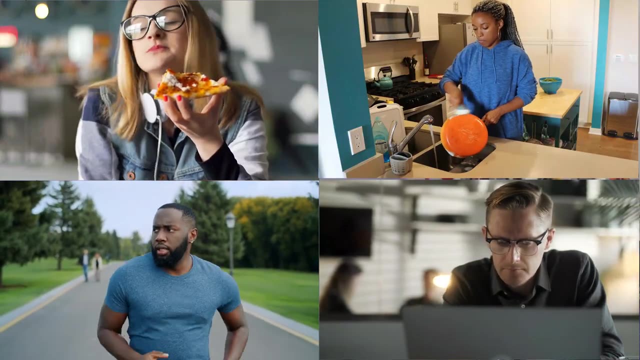 is ATUS or ATUS A-T-U-S- the American Time Use Survey. This is a data set where people keep track of what they do during the day, what kind of activities they're involved in, who they're with, And then you can match this with other data about that individual. 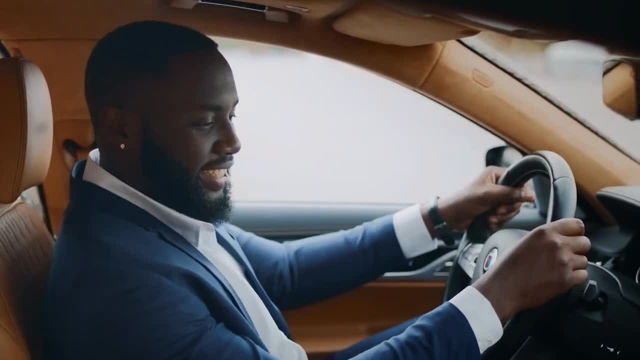 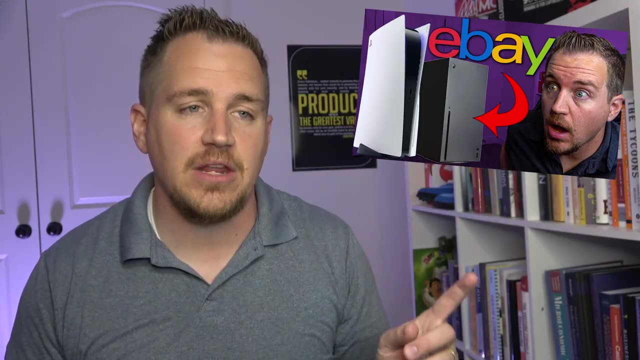 and learn about how income is related to how you spend time during your day or how people spend time with their children and what that leads to child outcomes. I use this in my video about the Xbox and the PlayStation and the relationship between income- employment. 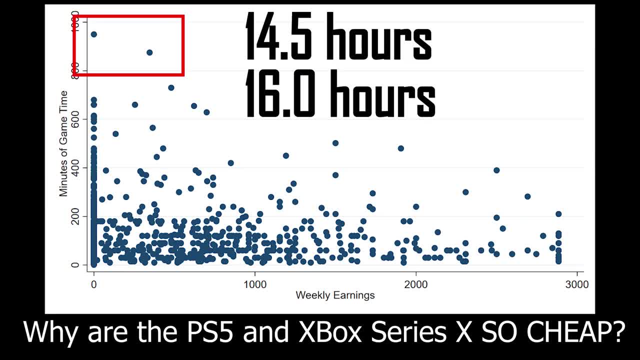 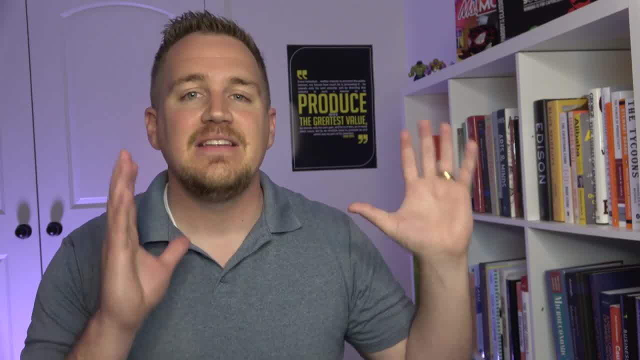 and how much time you spend playing video games. So I was able to just grab this data, do a quick analysis. Super interesting to look into Ipems and find data sets that look interesting to you. And there's also this really cool aspect of 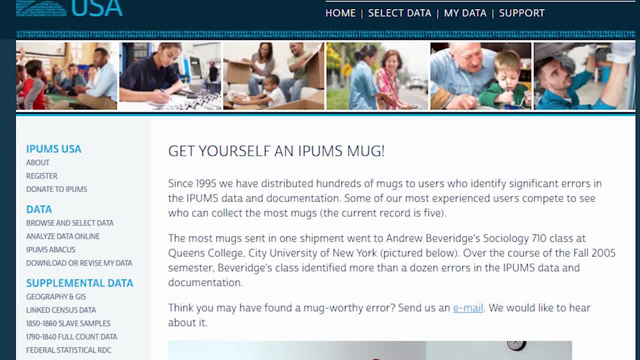 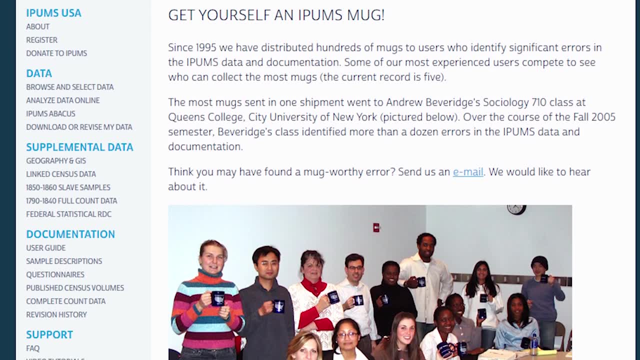 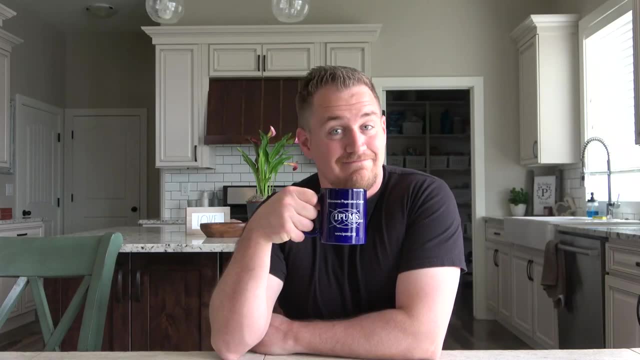 Ipems, where, if you find a mistake in their data, they'll actually send you this coffee mug as this trophy. And obviously, since it's such a popular data set, it's really hard to get one of these mugs, So you have to be just like one of the top economists to actually be awarded one of these. 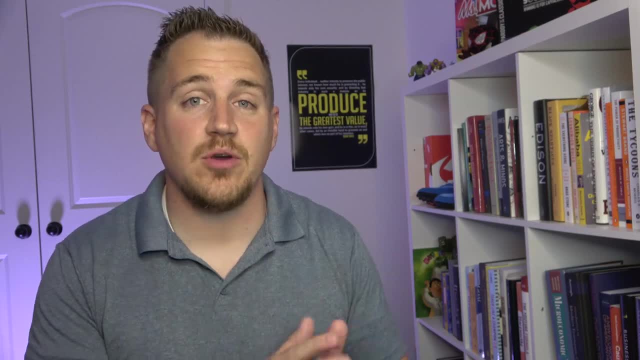 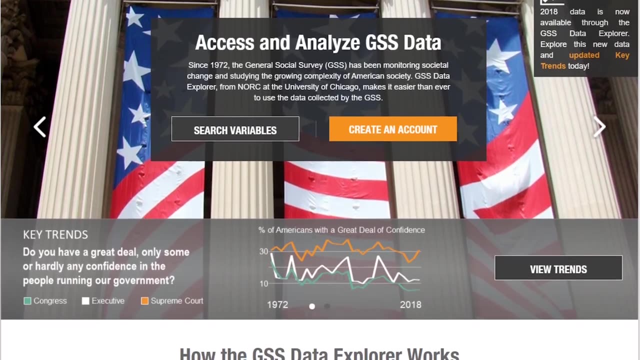 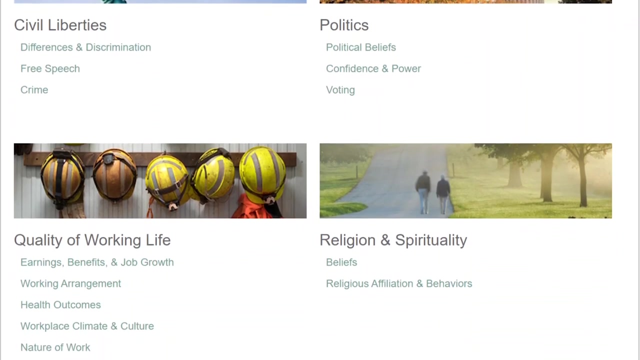 mugs. So the second data set that I recommend is the General Social Survey. This is a survey that's been done by the University of Illinois, asking questions about just general social issues. This could be opinions on civic liberties, on religious freedom, but it's also micro data on occupation. 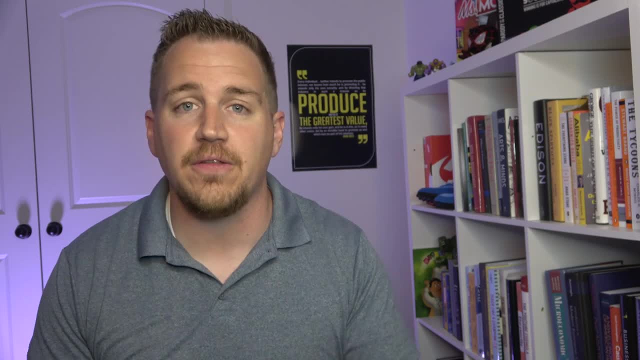 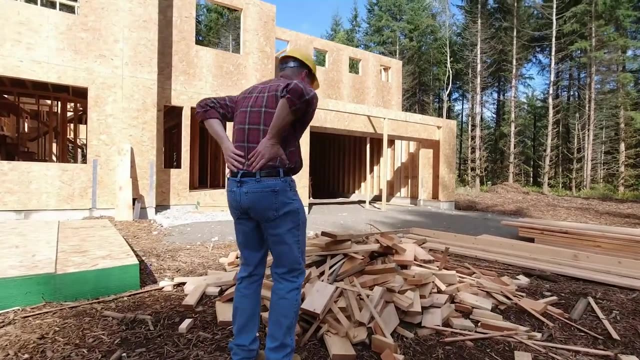 choice and health. So let's say you were interested in the relationship between education and health. You could look at indicators on education and then look at how it's related to back pain is one of the questions in here. You could look at how different people trust their 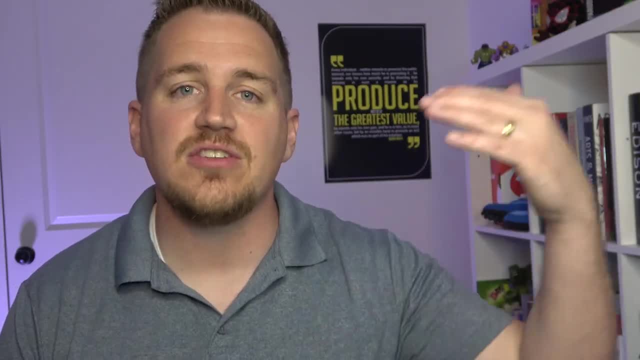 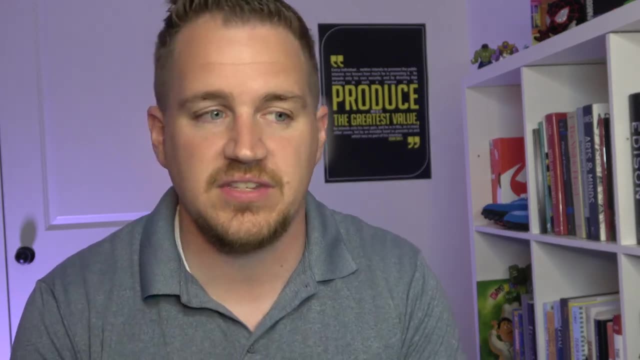 country. There are a ton of questions here. You can see how these are evolving over time. You can see how they're evolving over space. But the best part about this is that you get to see four individuals, somebody who doesn't trust Congress. What are their other attributes? Is this somebody? 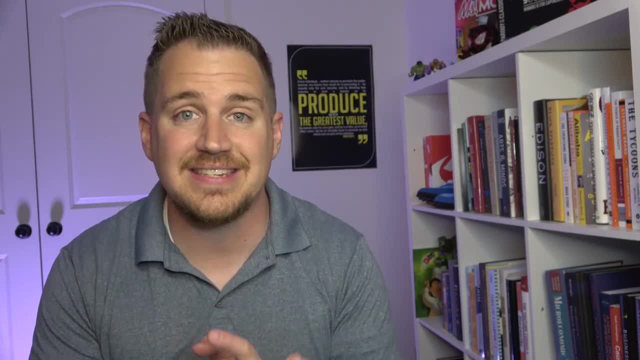 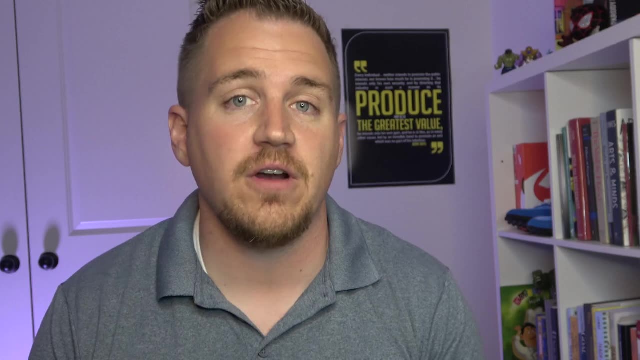 more or less educated? Is this somebody more or less likely to live in certain states? You can really dive into some interesting, fascinating questions. In fact, if you are doing an econometrics project for an undergraduate research class, I highly recommend going to 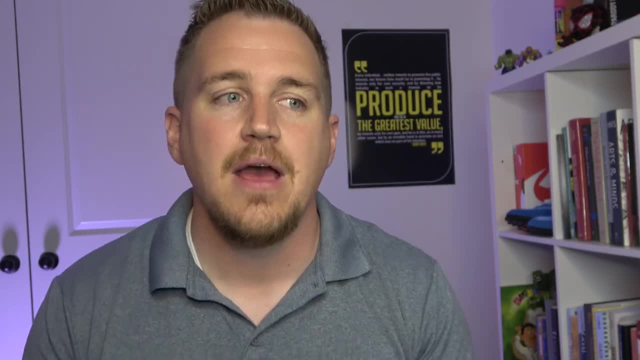 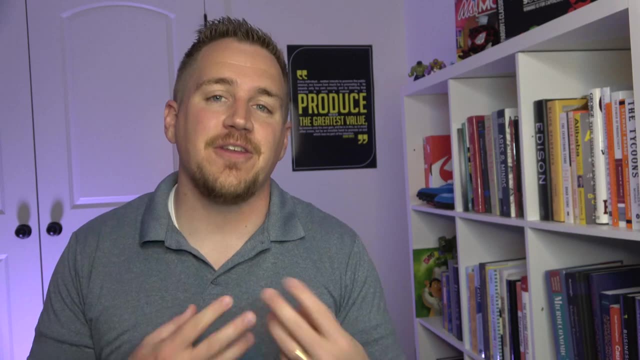 GSS and looking through the questions that they ask, because you might find something that's way more interesting than a boring economics question that you're just not interested in. The third data set I want to bring up is the demographic and health survey. This is kind of like the GSS, but it's much more limited in the questions that they ask. They're really focused on health questions, demographics, a few other questions, But then the question is: why would you want something that has fewer questions asked? Well, the answer is that they. 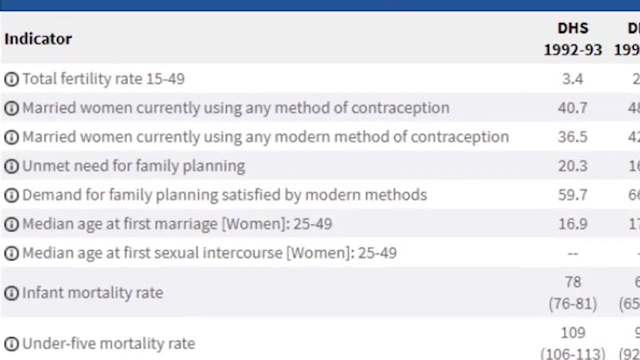 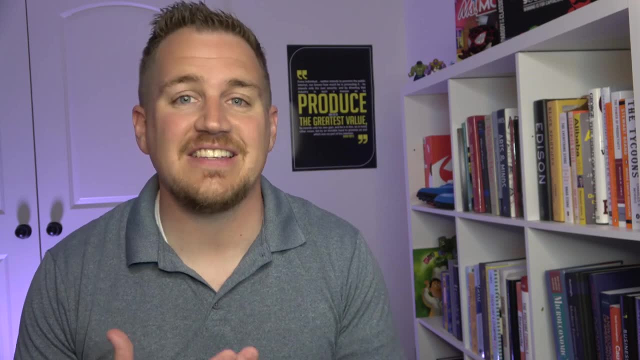 ask this around the world, and especially in developing countries. So if you're interested in development economics, this should be one of the first data sets that you go to. These are all data sets that are going to help you with research If you want to understand. 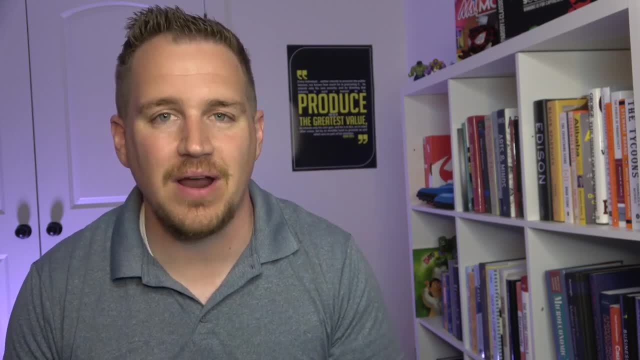 why you should be involved in research. go ahead and check out this video right here.